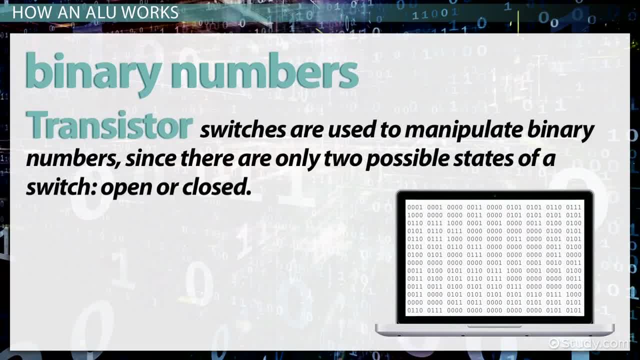 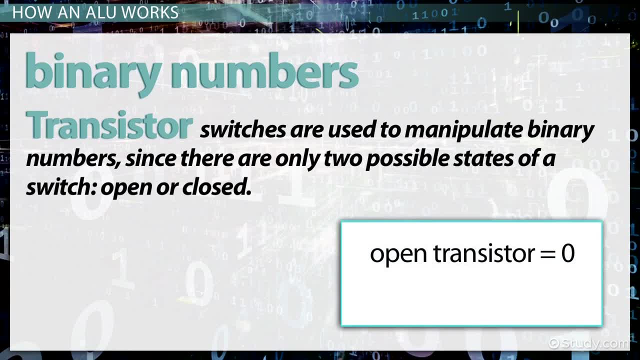 switches are used to manipulate binary numbers, since there are only two possible states of a switch: open or closed. an open transistor through which there is no current represents a zero. a closed transistor through which there is a current represents a one. operations can be accomplished by connecting multiple transistors. 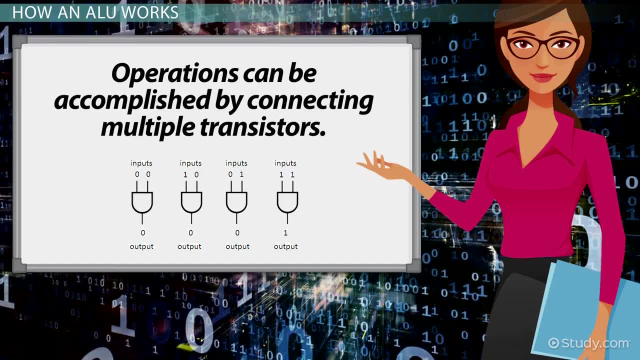 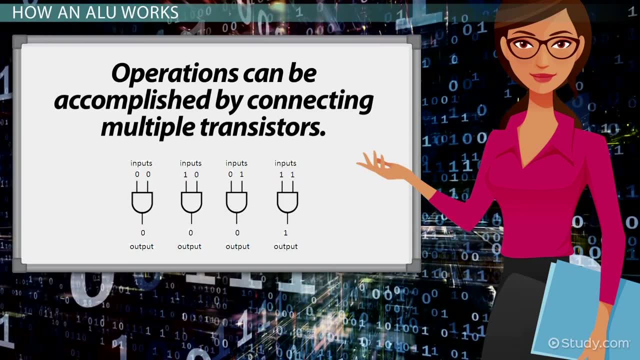 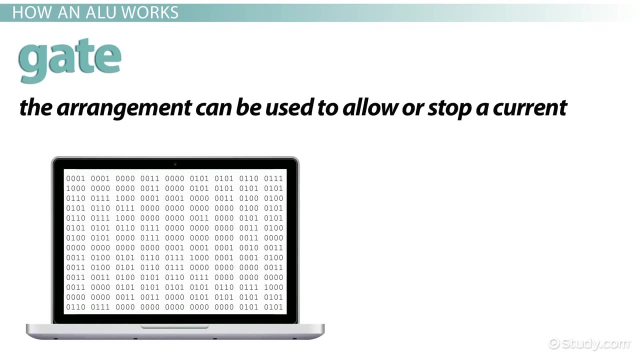 one transistor can be used to control a second one and effect turning the transistor switch on or off depending on the state of the second transistor. this is referred to as a gate because the arrangement can be used to allow or stop a current. the simplest type of operation is a not gate. this uses only a single. 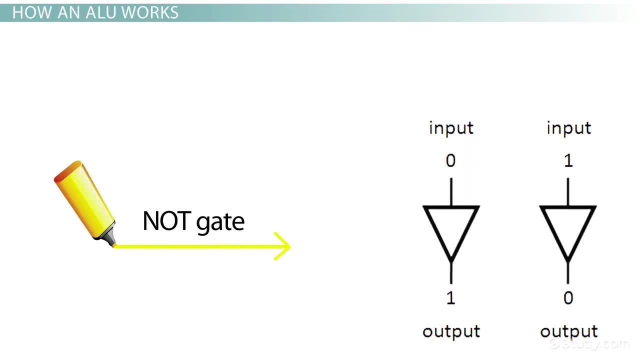 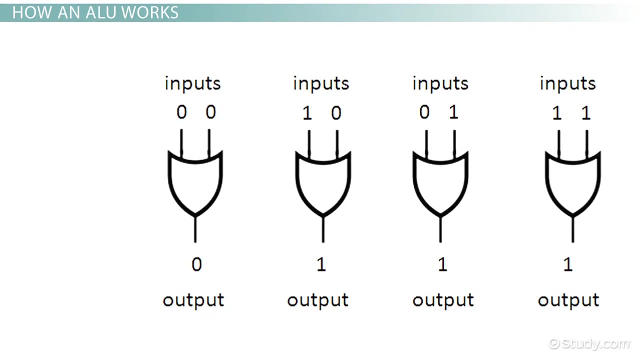 transistor. it uses a single input and produces a single output, which is always the opposite of the input and output. This figure shows the logic of the NOT gate, how a NOT gate processes binary data. Other gates consist of multiple transistors and use two inputs. 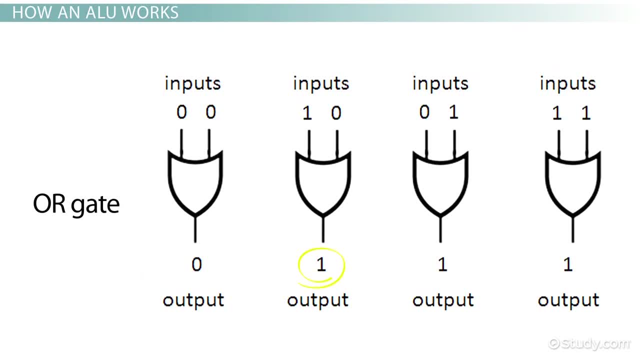 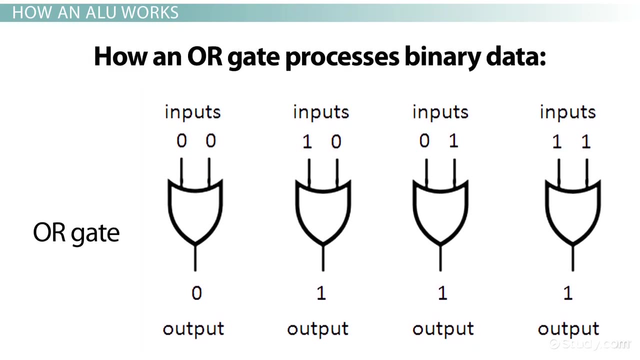 The OR gate results in a 1 if either the first or the second input is a 1.. The OR gate only results in a 0 if both inputs are 0.. This figure shows the logic of the OR gate: how an OR gate processes binary data. 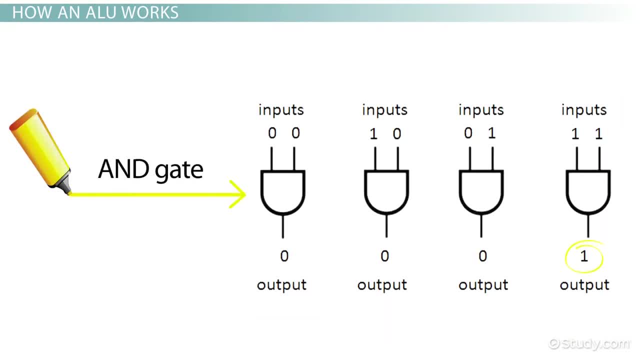 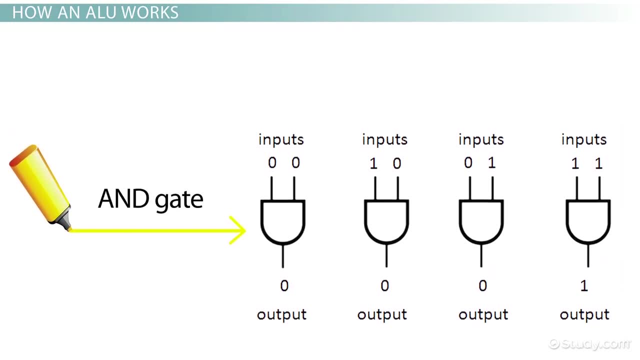 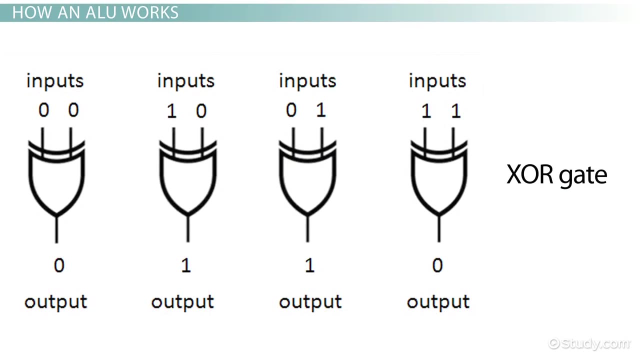 The AND gate results in a 1 only if both the first and second input are 1s. This figure shows the logic of the AND gate, how an AND gate processes binary data. The XOR gate, also pronounced XOR gate, results in a 0 if both the inputs are 0 or if both are 1.. 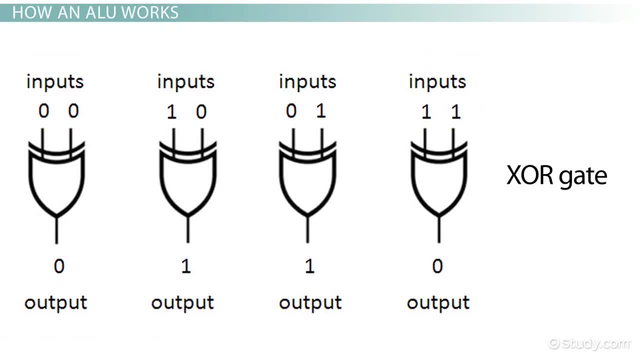 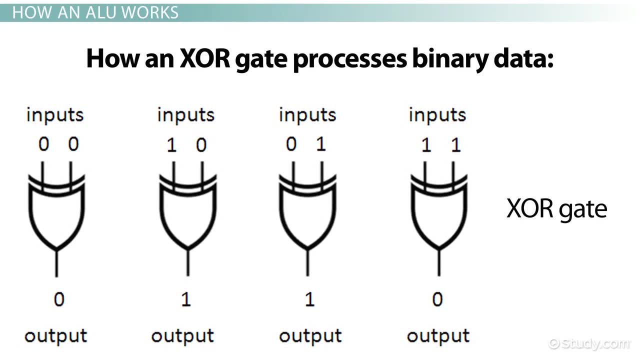 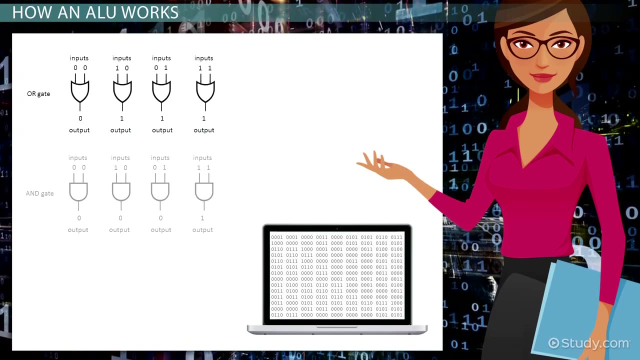 Otherwise the result is a 1.. This figure shows the logic of the AND gate, how a XOR gate processes binary data. The various gates sound a little abstract, but remember that a computer only processes binary data. When you follow the binary logic of these operations, 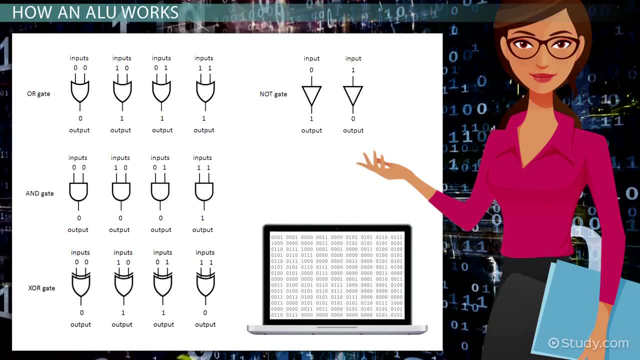 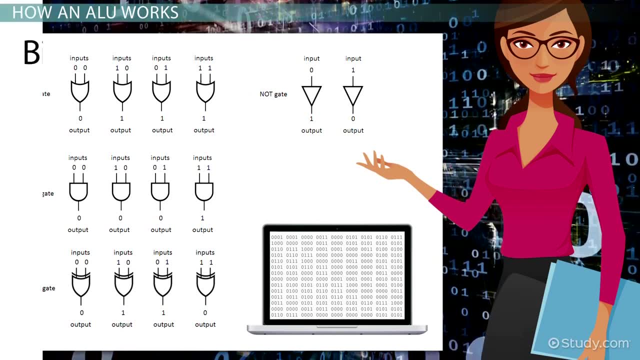 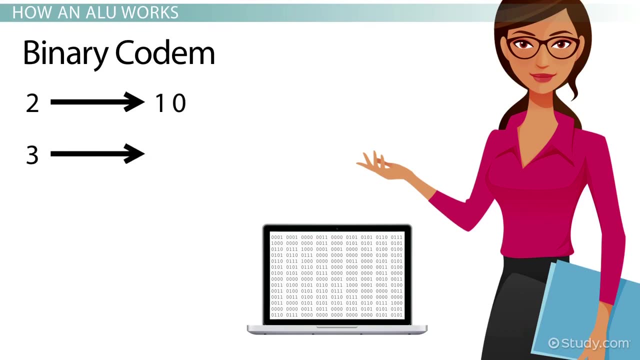 you are starting to think like a computer. Different combinations of the logic gates make it possible to perform arithmetic operations. For example, in binary codem the number 2 is represented as 10, and the number 3 is represented as 11..